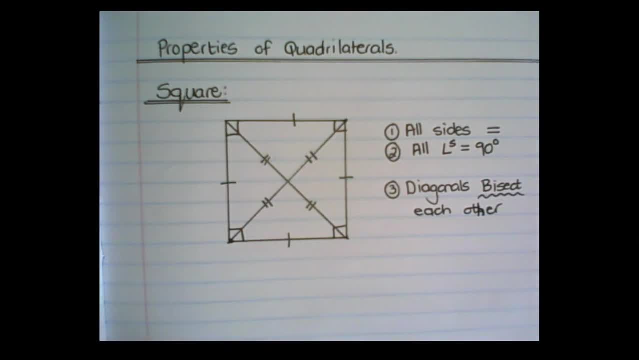 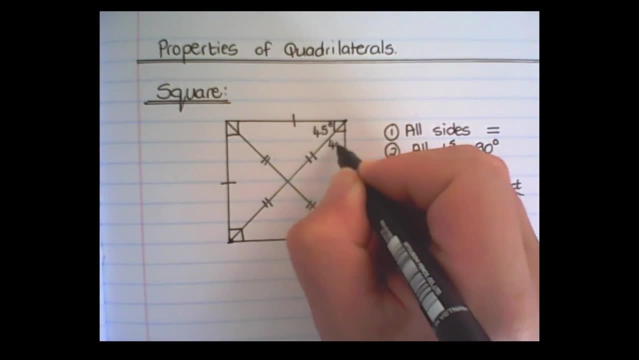 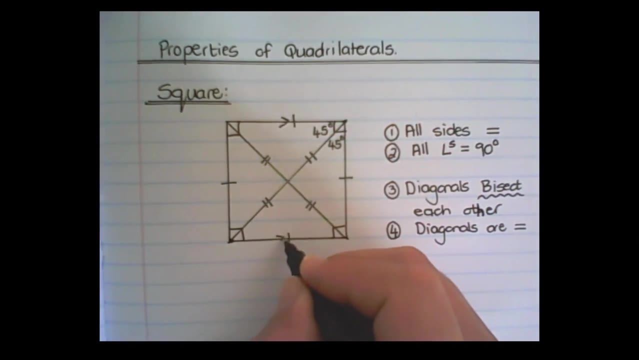 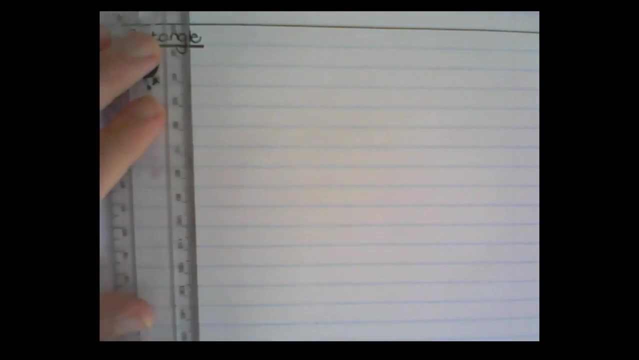 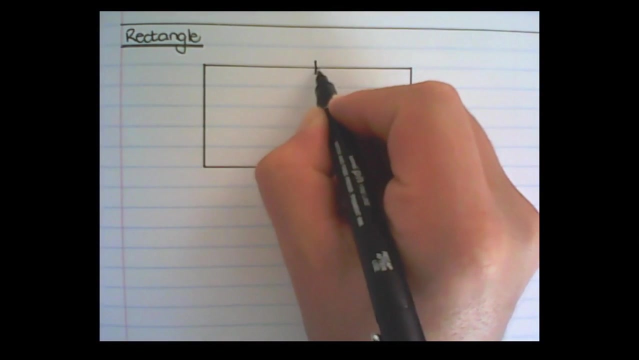 of the halves would be equal in length, With the diagonals cutting each other in half. the corners are also bisected And, lastly, opposite lines of a square are parallel to each other. Next, we have a rectangle. What we know from rectangles are the opposite. 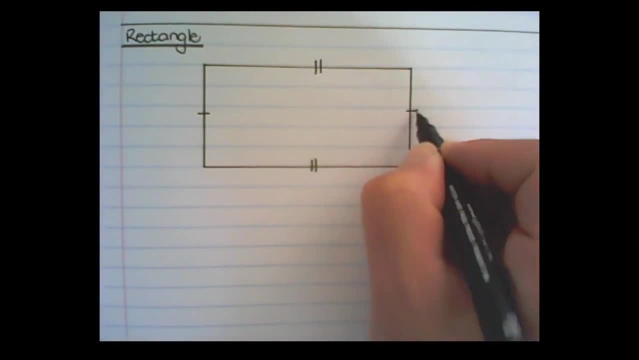 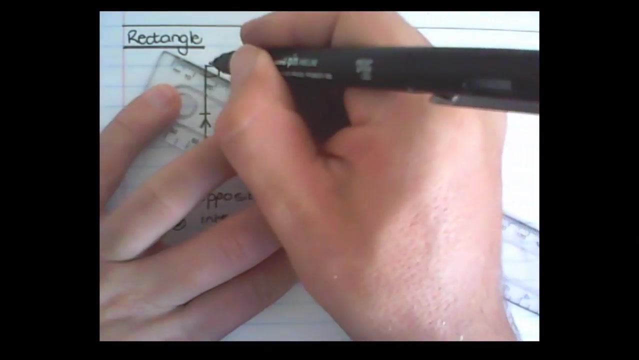 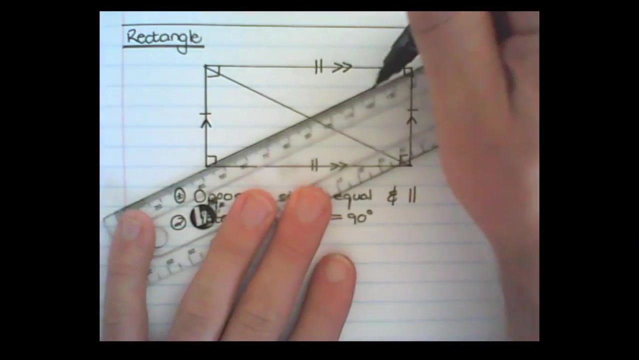 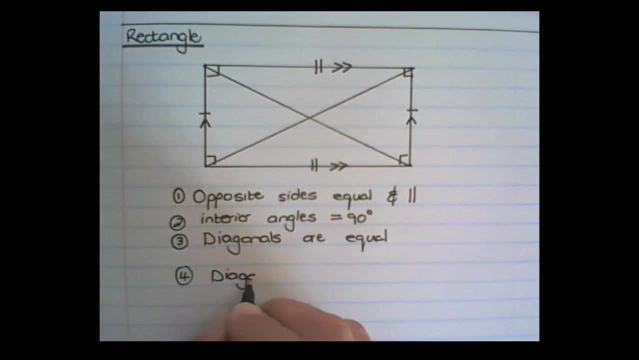 sides are of equal length and the opposite sides are parallel. We also know that all interior angles are 90 degrees, The diagonals, meaning the lines running from corner to corner, are equal in length, and that diagonals bisect each other, Meaning they cut each other in half. What we can see with these lines are that the lines 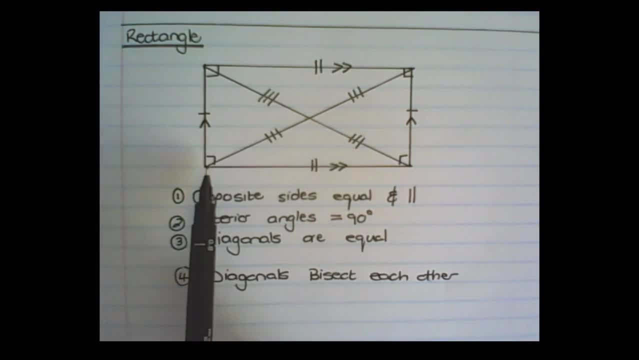 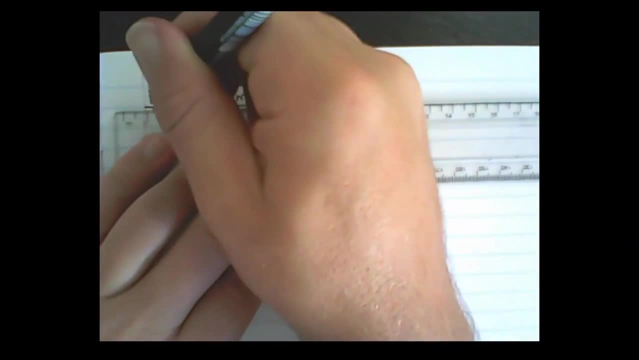 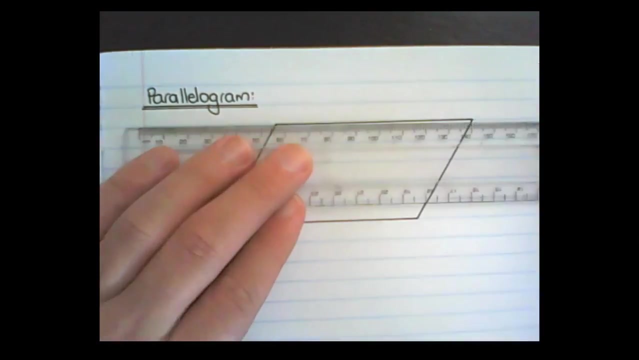 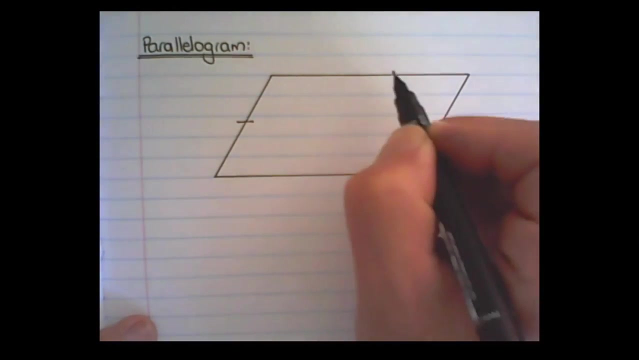 from this diagonal to the center and all of the other diagonals to the center are equal in length. The next quadrilateral is the parallelogram. What we know about the parallelogram is that the opposite sides are equal in length and the opposite sides are parallel, And we indicate the parallel with arrows. 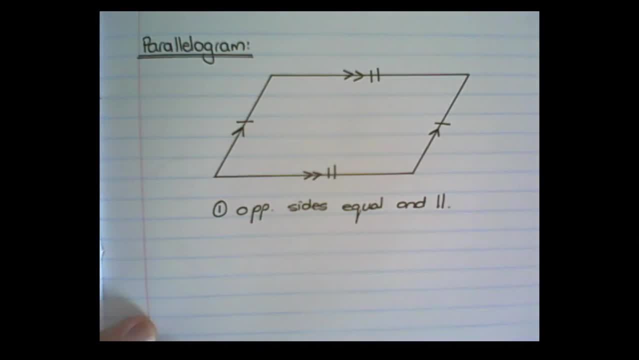 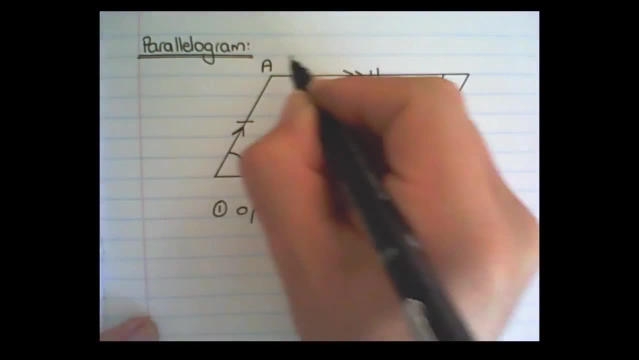 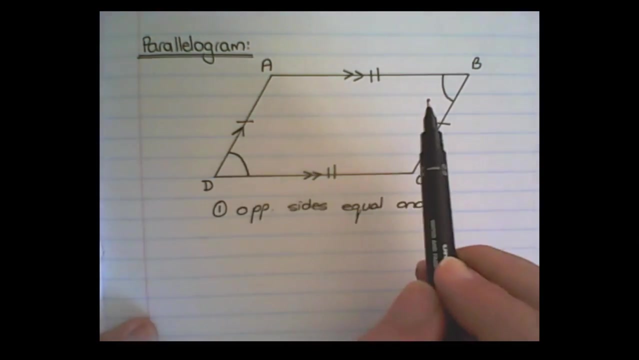 The interior angles are not all the same, but the opposite angles are equal in size, Meaning. I have a parallelogram: ABCD, angle D would be equal to angle B and angle A would be equal to angle C. Now, if I draw a diagonal, 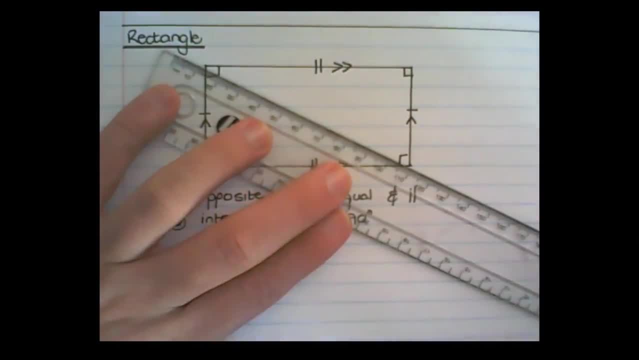 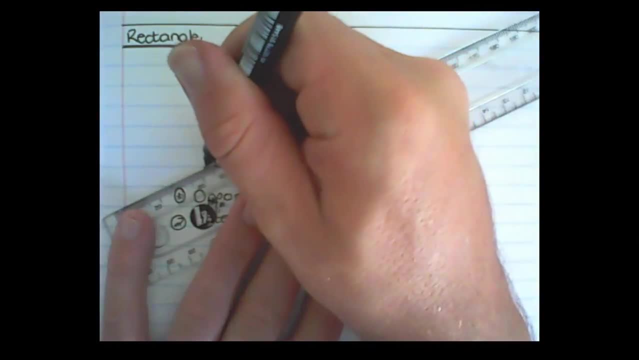 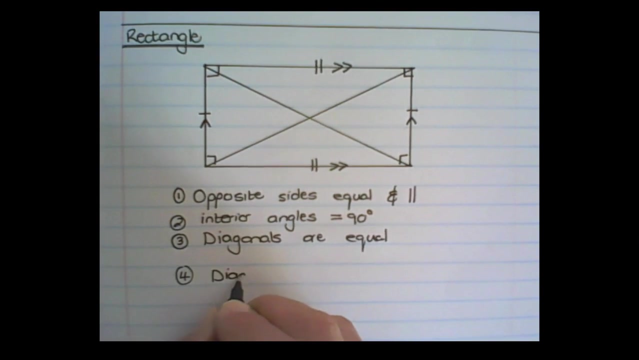 The diagonals, meaning the lines running from corner to corner are equal in length, And that diagonals bisect each other, meaning they cut each other in half. What we can see with these lines are that the lines from this diagonal to the center and all of the other diagonals to the center 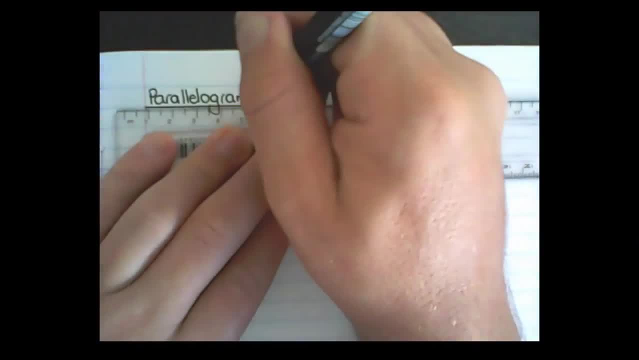 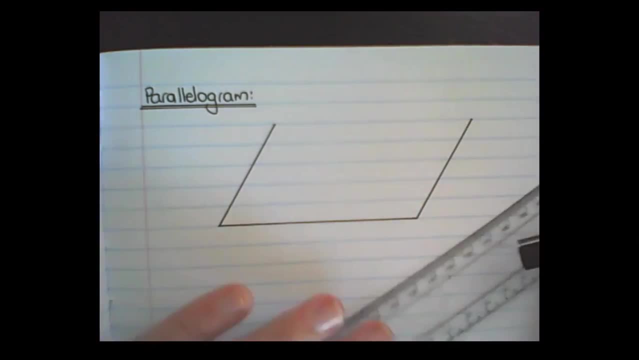 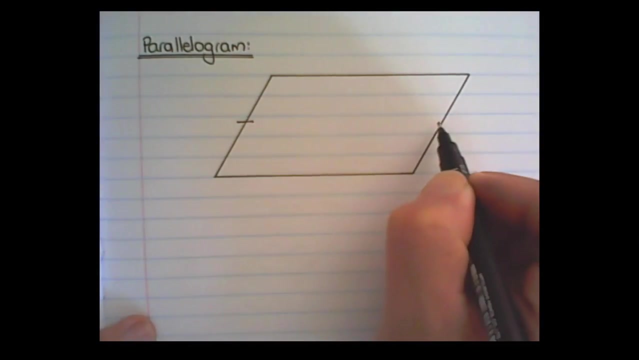 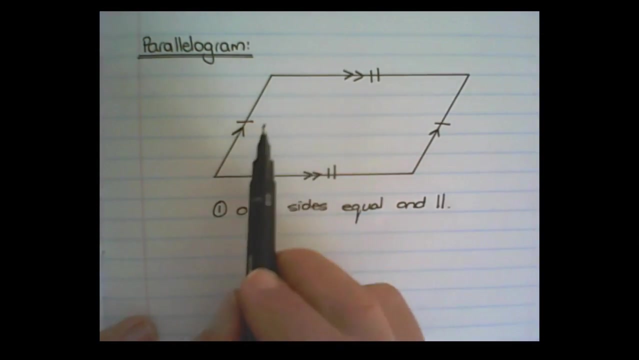 are equal in length. The next quadrilateral is the parallelogram. What we know about the parallelogram is that the opposite sides are equal in length And the opposite sides are parallel. We indicate parallel with arrows. Now, the interior angles are not all the same, but the opposite angles are equal in size. 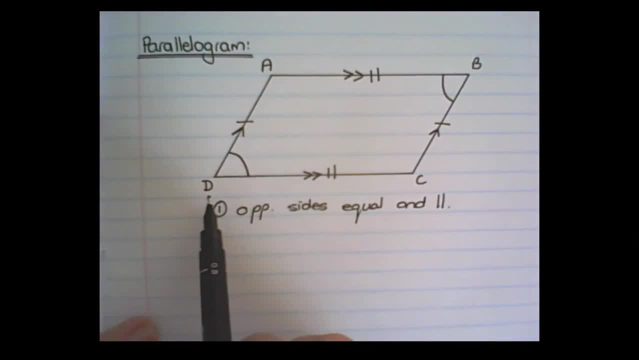 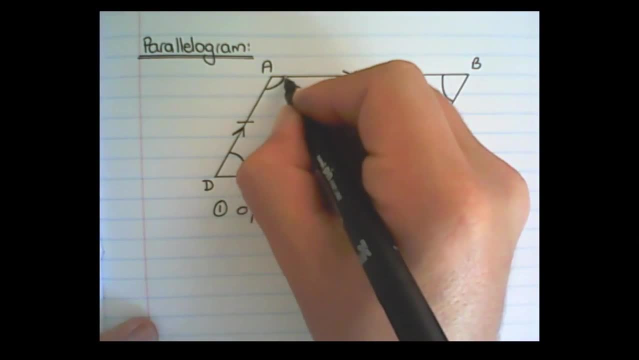 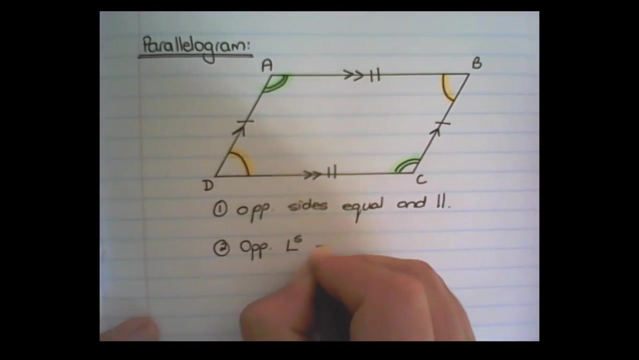 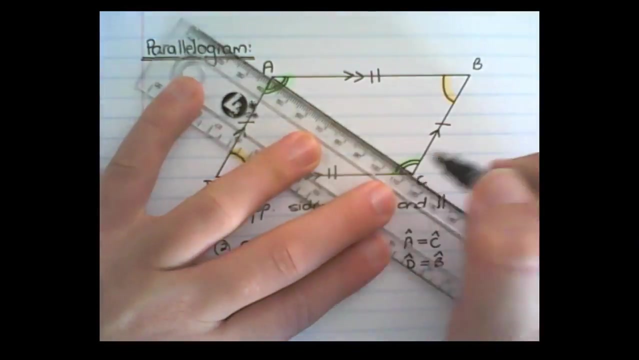 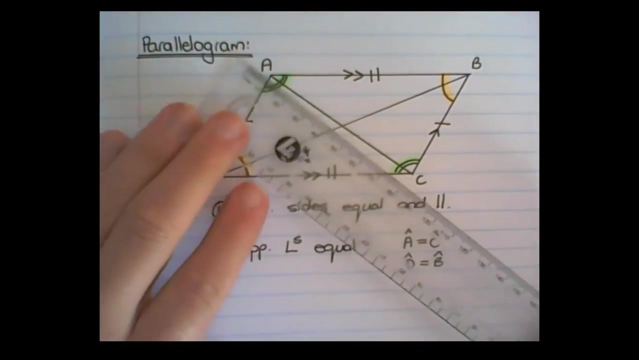 Meaning, if I have a parallelogram ABCD, angle D would be equal to angle B and angle A would be equal to angle C. Now if I draw a diagonal and another diagonal, they are not equal in length. I would see that the one diagonal is shorter than another. 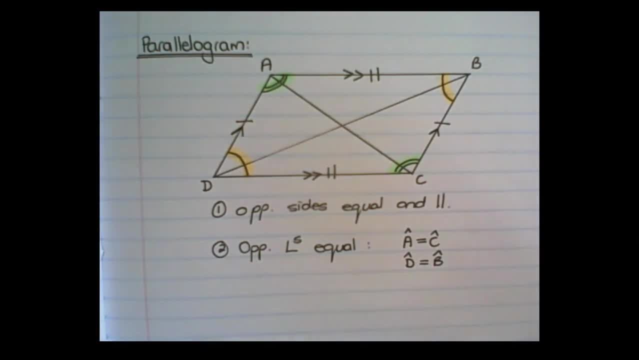 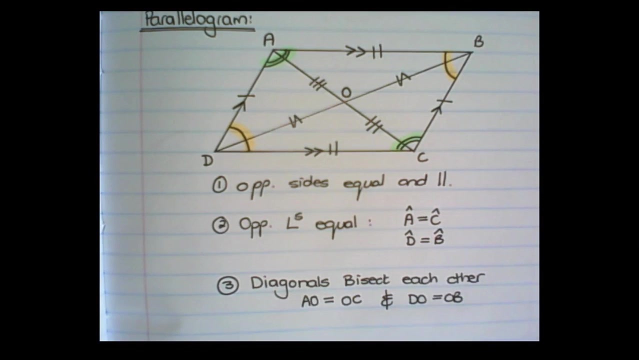 diagonal. But what diagonals do is they bisect each other, meaning they cut each other in half. So this diagonal cuts the line AC in half, meaning the line AO would be equal to OC, and the line AC cuts DB in half, meaning the line DO would be equal to line OB. You can also find properties of parallel. 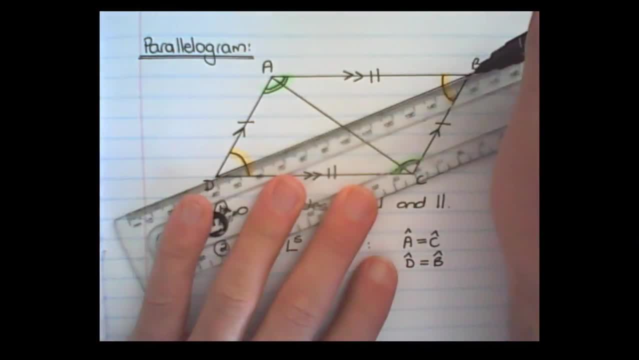 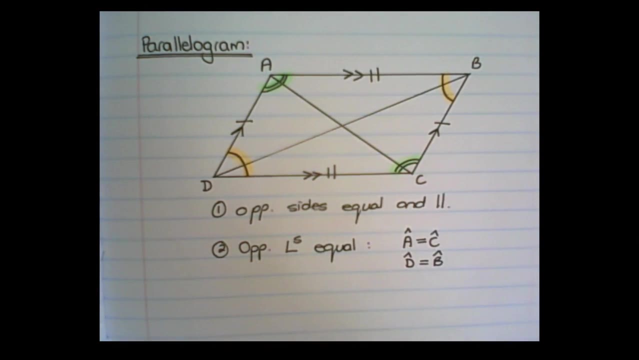 and another diagonal. they are not equal in length. I would see that the one diagonal is shorter than another diagonal. but what diagonals do is they bisect each other, meaning they cut each other in half. so this diagonal cuts the line AC in half. 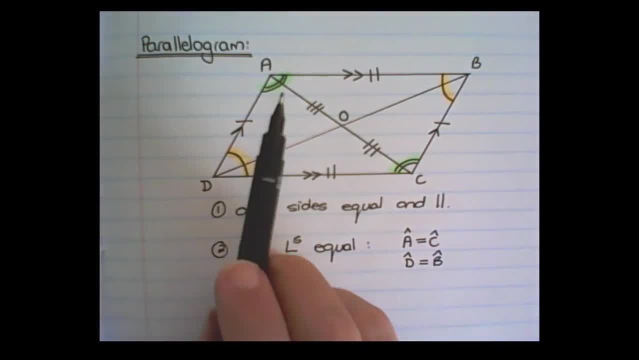 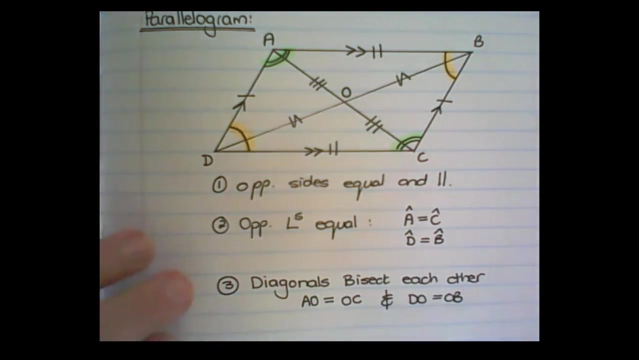 Meaning the line AO would be equal to OC and the line AC cuts DB in half, Meaning the line DO would be equal to line OB. You can also find properties of the diagonal line A and the diagonal line B. You can also find properties of parallel lines. 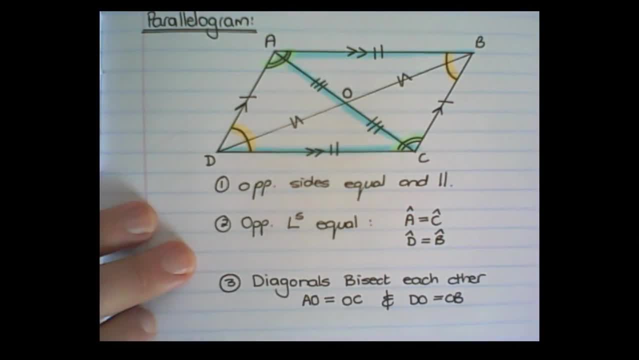 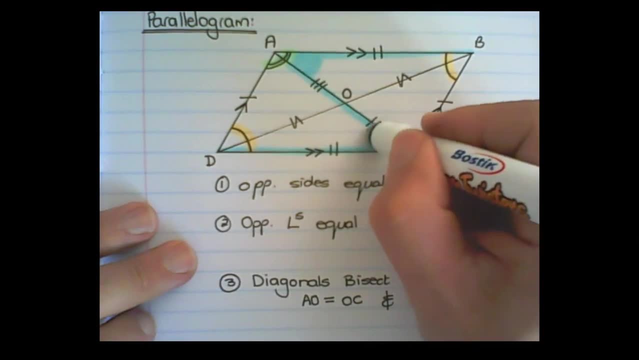 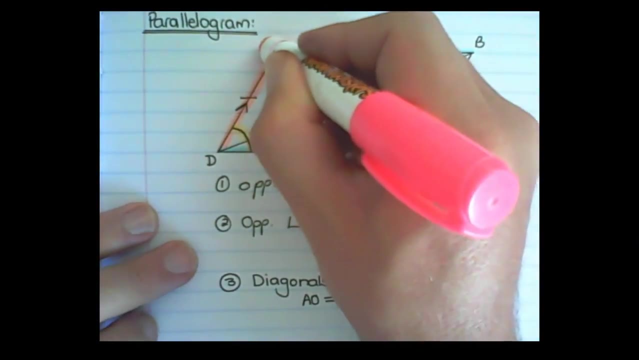 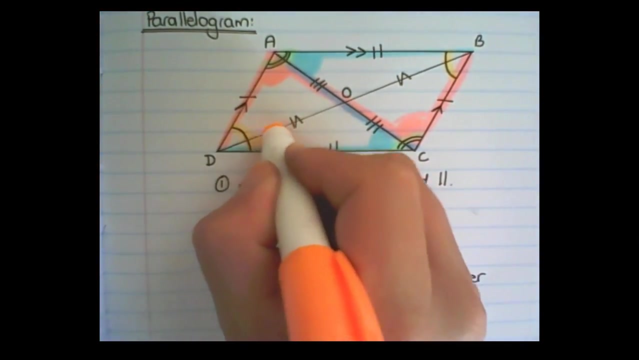 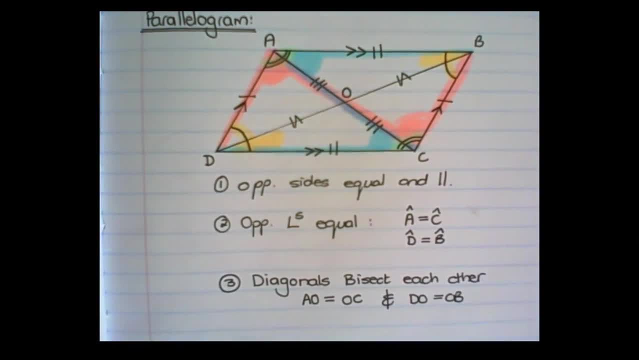 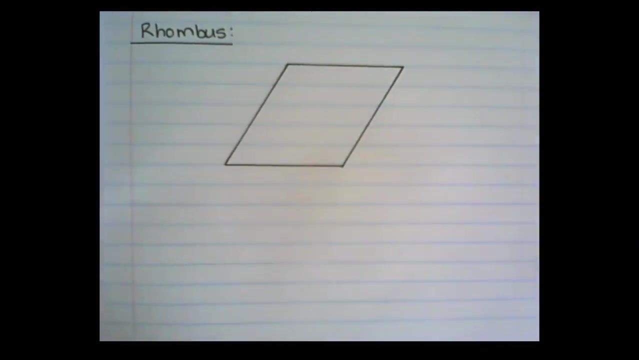 So be careful when you work with a parallelogram that you're not getting confused of which angle is the most important To. The next figure is called a rhombus. With a rhombus, the opposite sides are all equal in length. 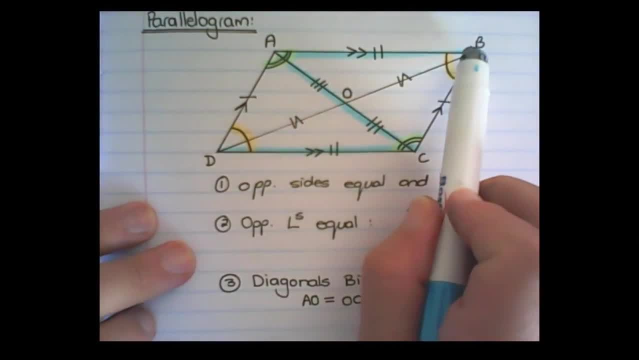 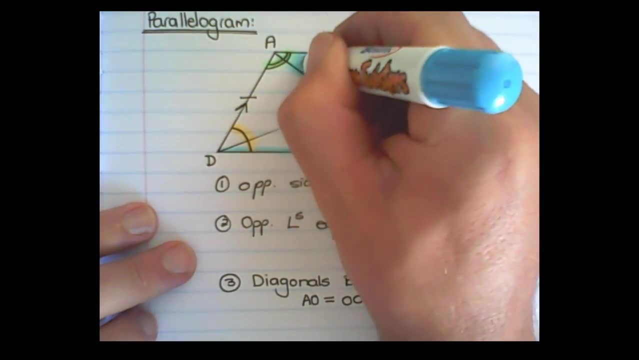 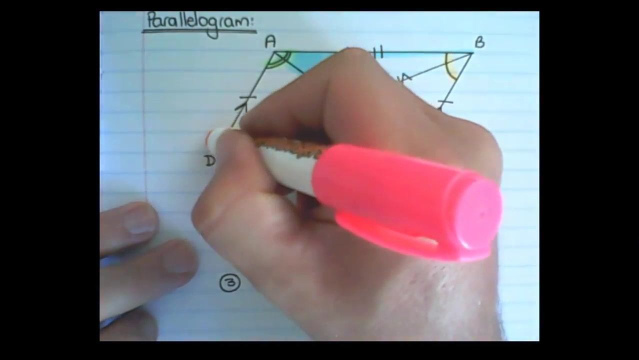 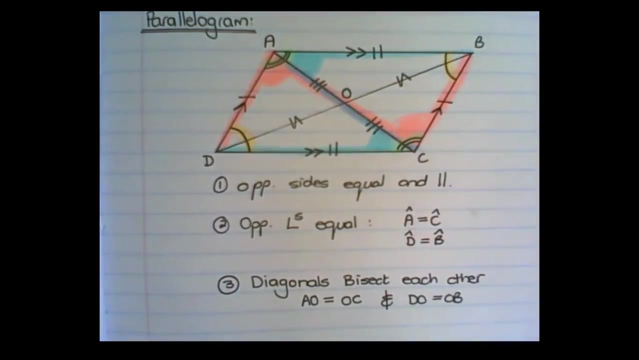 lines. If I look at what I have highlighted, I can see alternate angles, meaning this angle inside would be equal to that angle, And other forms of alternate angles exist throughout the whole parallelogram. So be careful when you work with a parallelogram that you're not getting confused of which. 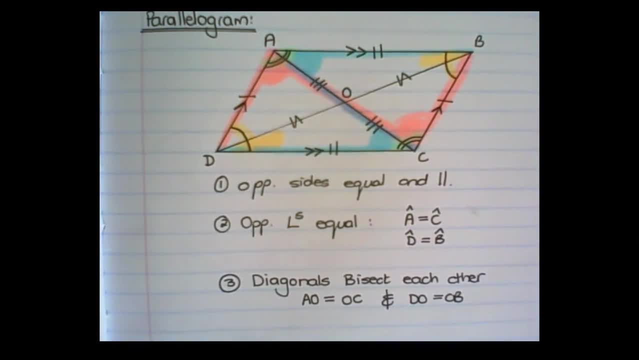 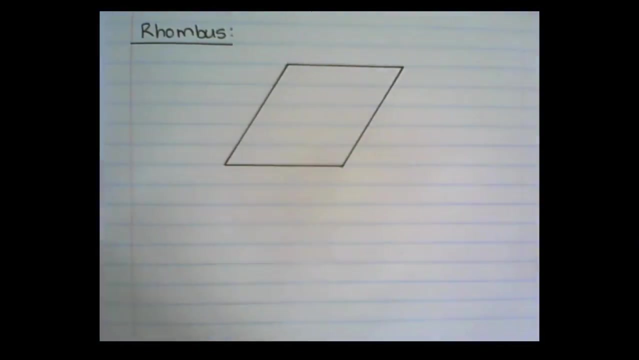 angles are equal to which. Don't try and memorize them, simply use what you have learned up until now. The next figure is called a rhombus. With a rhombus, the opposite sides are all equal in length, So that is the main property of a rhombus. 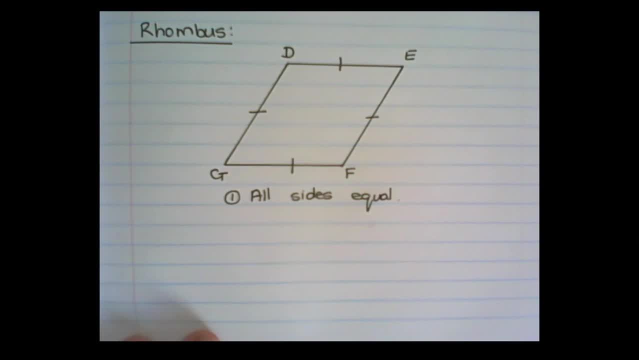 So all sides are equal. Opposite sides of the rhombus are parallel And it has the same properties as a parallelogram with opposite angles: equal meaning: angle E is equal to angle G and angle D is equal to angle F. 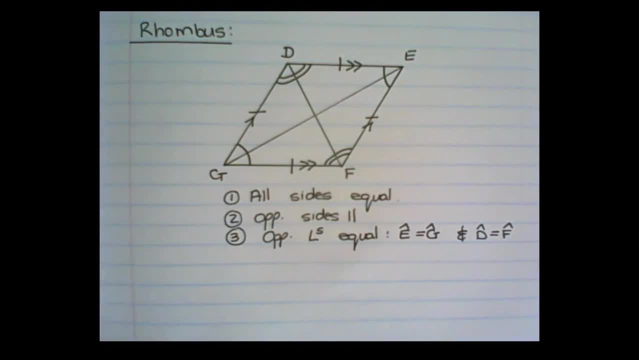 The diagonal cuts the line AC in half, meaning they cut each other in half, meaning the line DO would be equal to angle F. The next figure is called a rhombus. With a rhombus, the opposite sides are all equal in length, So that is the main property of a rhombus. 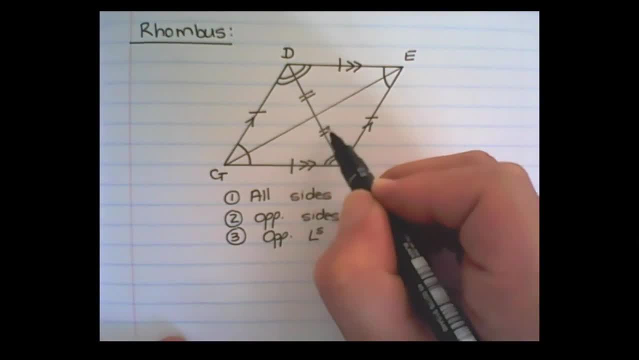 The next figure is called a rhombus. With a rhombus, the opposite sides are all equal in length. So that is the main property of a rhombus. So a rhombus has diagonal lines bisecting each other. 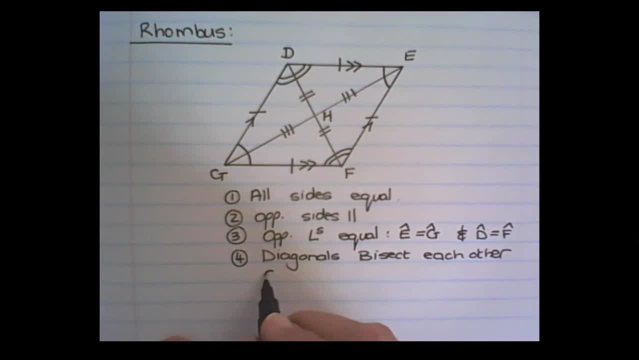 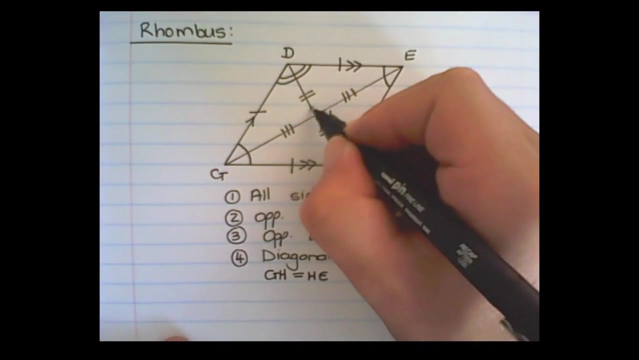 Roger, Meaning the line GH would be equal to HE And the line DH would be equal to line HF. And another big property of a rhombus is diagonal bisects at 90 degrees. So this means a rhombus has diagonal bisects at 90 degrees. 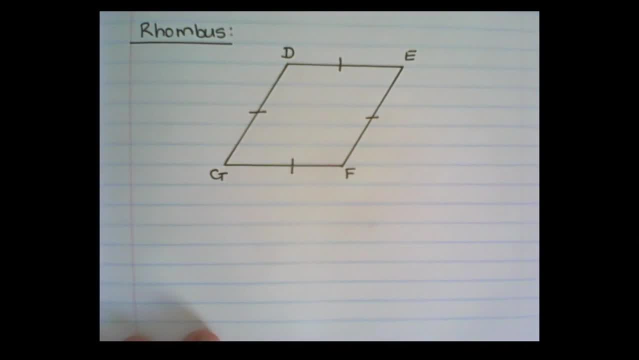 So that is the main property of a rhombus. So all sides are equal. Opposite sides of the rhombus are parallel And it has the same properties as a parallelogram with opposite angles equal Meaning. angle E is equal to angle G. 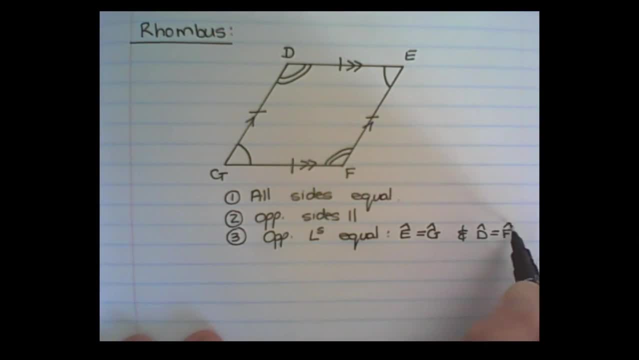 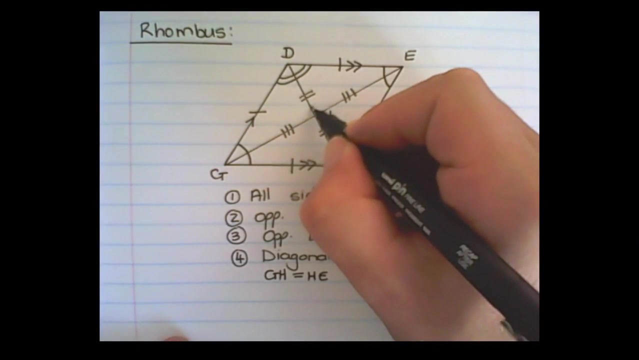 And angle B is equal to angle C And angle D is equal to angle F. Diagonal lines bisect each other, Meaning that the line GH would be equal to HE And the line DH would be equal to the line HF. And another big property of the rhombus is diagonals bisect at 90 degrees. 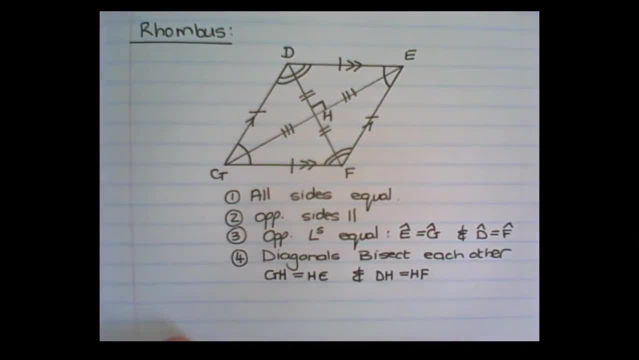 So the line at which they cut each other is 90 degrees. So the two main properties of a rhombus are: all sides are equal in length And diagonals bisect at 90 degrees. They can be cut at 90 degrees. enter is equal to whatever is at 90 degrees each side. 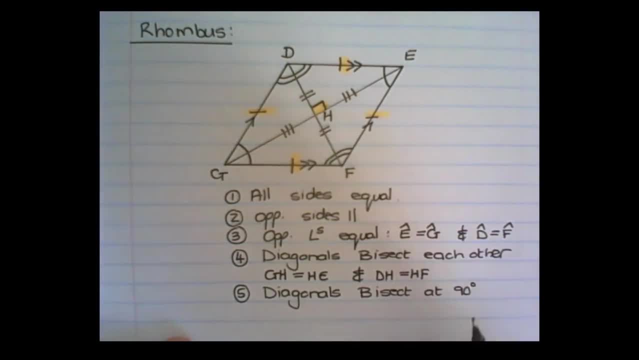 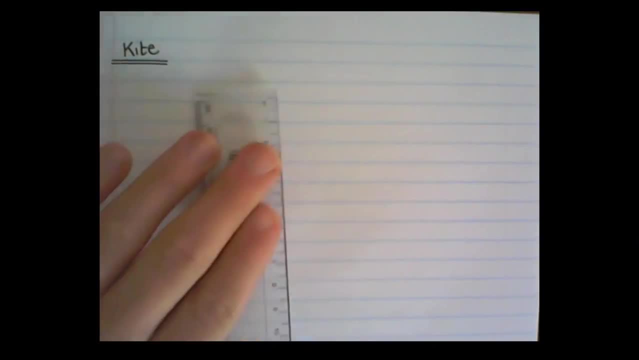 Withめging Grid, line W is equal to diet 1, or 3.. And the line Q is equal to diagonals bisect. one of the PelManx And diagonals bisect will equal Quadruped 1, or 4.. 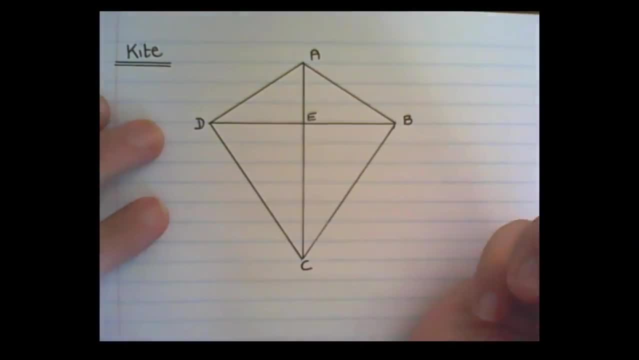 So it is equal to the tangent of all sides of the big bangeth. What is the solution for this? up to digital? So our second figure is a kite kite. the diagonals of the quadrilateral meet at 90 degrees, And a nice word for 90 degrees. 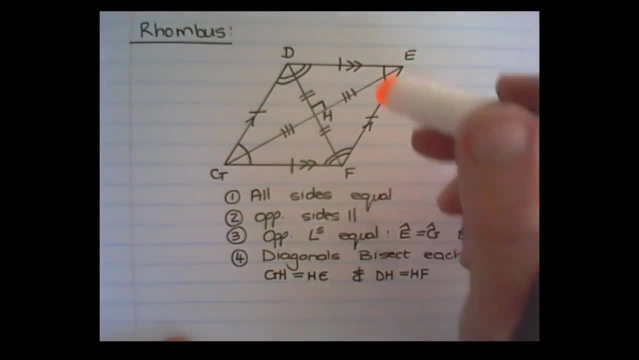 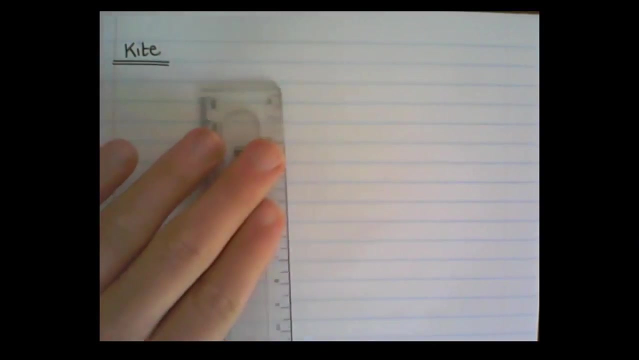 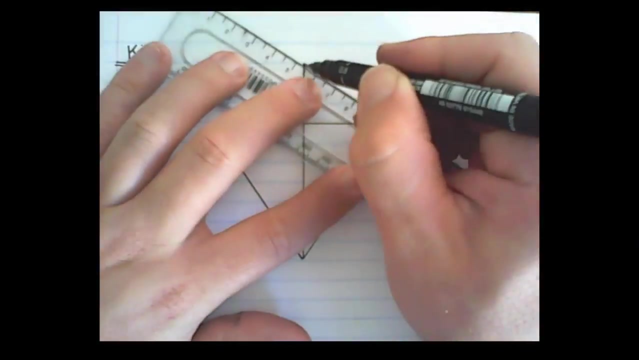 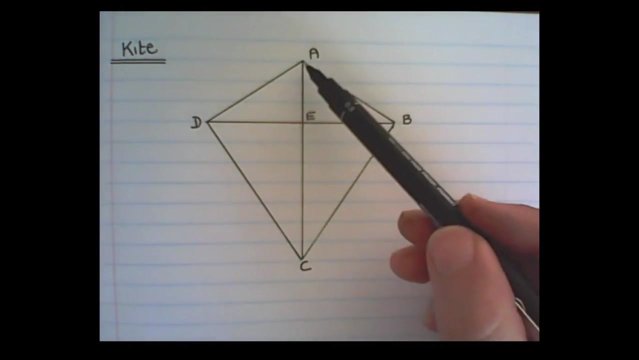 at which they cut each other is 90 degrees. so the two main properties of a rhombus are: all sides are equal in length and diagonals bisect at 90 degrees. you, our second last figure is a kite. so with a kite, the diagonals of the quadrilateral meet at 90 degrees. 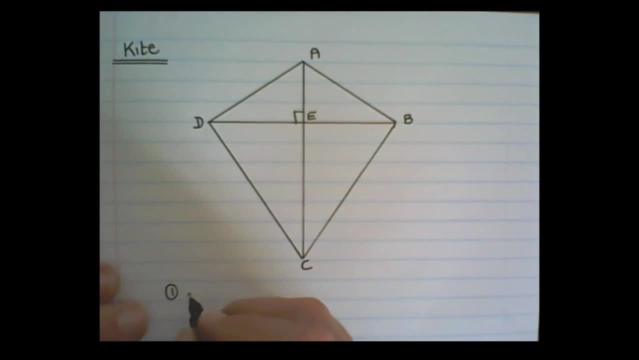 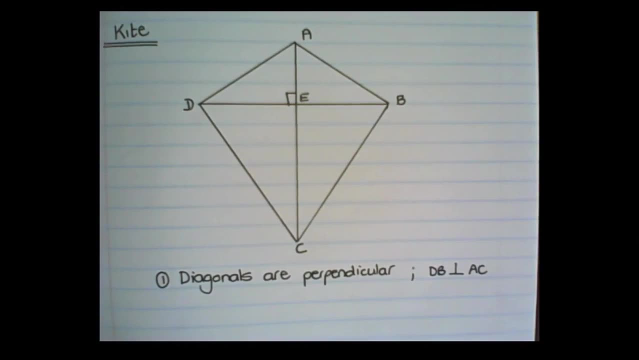 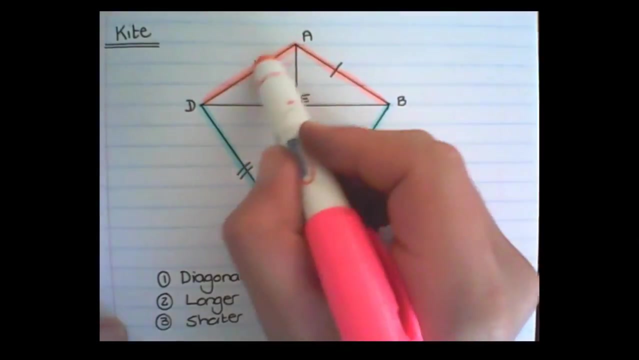 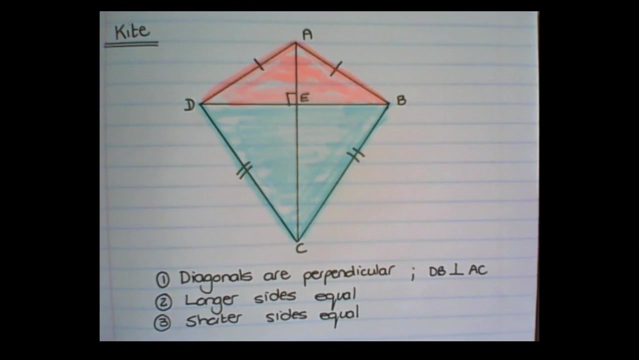 and the- a nice word for 90 degrees- is perpendicular. another property of a kite is that the longer sides are equal in length and the shorter sides are equal in length. there are no parallel sides in the kite, but what we can see is that we have two. 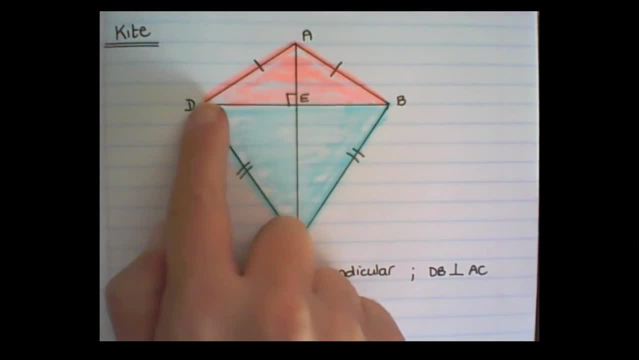 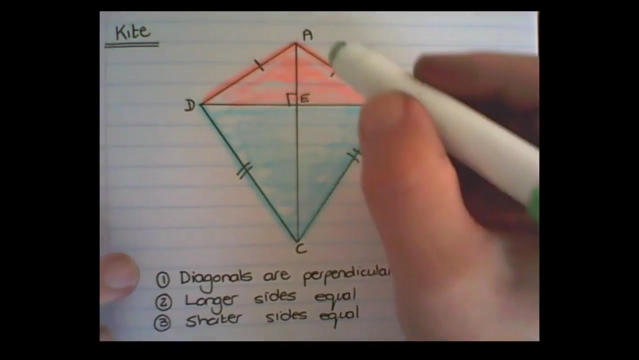 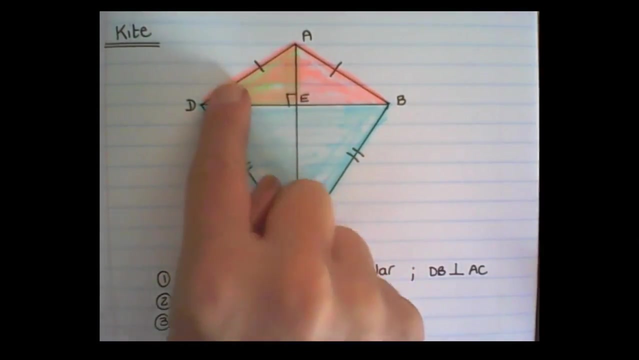 isosceles triangles. so if I combine those two triangles I have one big isosceles triangle, and if I combine the two blue triangles I have an isosceles triangle. another strong feature of a kite is that we can use pythagoras to solve sides or lengths of sides in the kite. 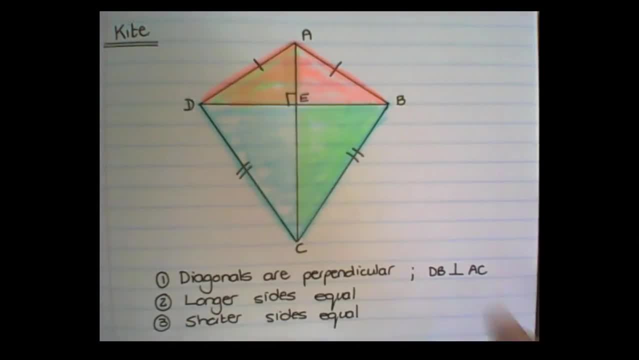 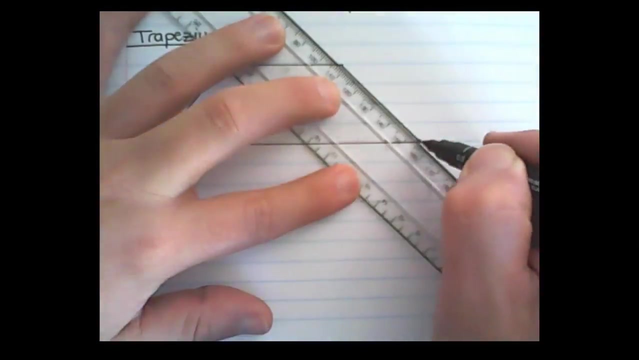 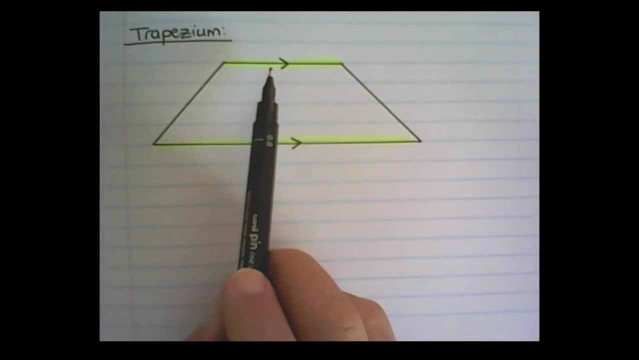 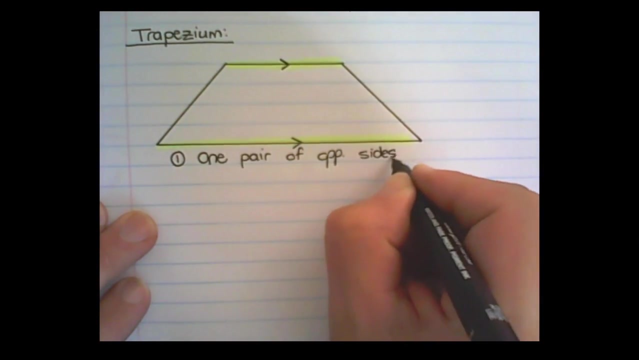 I can apply pythagoras here, because this angle is vertically opposite from that one and therefore also equal to 90 degrees. our last figure is a trapezium, and it only has one property, property, that is, that one pair of opposite sides are parallel.